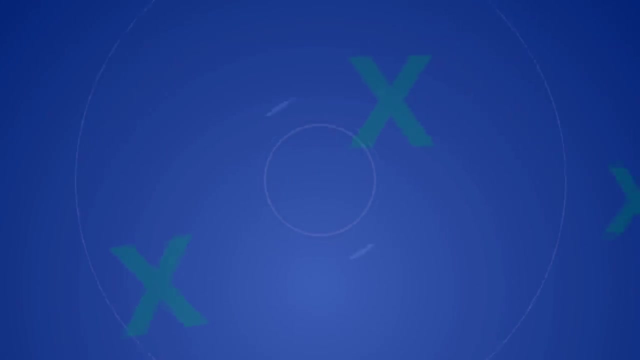 1 x 1 is 1.. 1 x 2 is 2.. 1 x 3 is 3.. Multiply by 1.. 1 x 4 is 4.. 1 x 5 is 5.. 1 x 6 is 6.. Multiply by 1.. 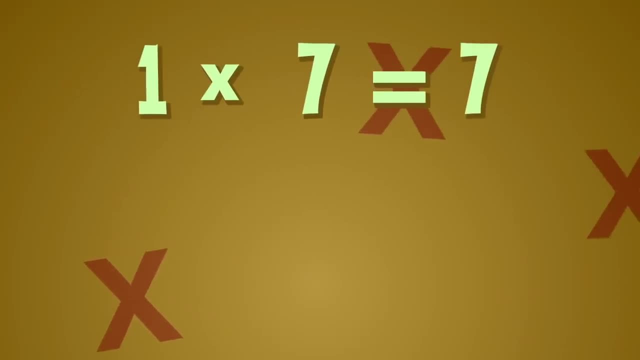 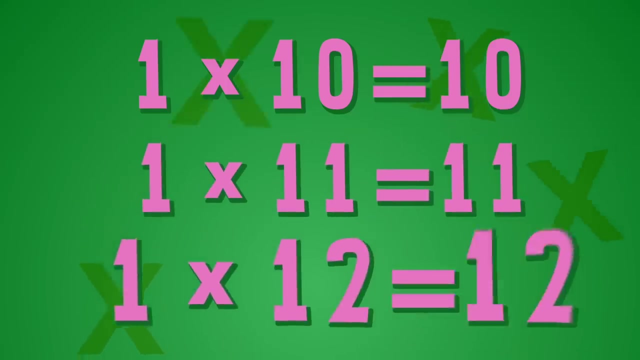 1 x 7 is 7.. 1 x 8 is 8.. 1 x 9 is 9.. Multiply by 1.. 1 x 10 is 10.. 1 x 11 is 11.. 1 x 12 is 12.. Multiply by 1.. 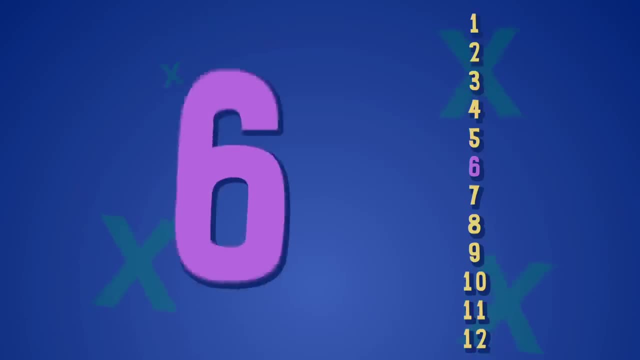 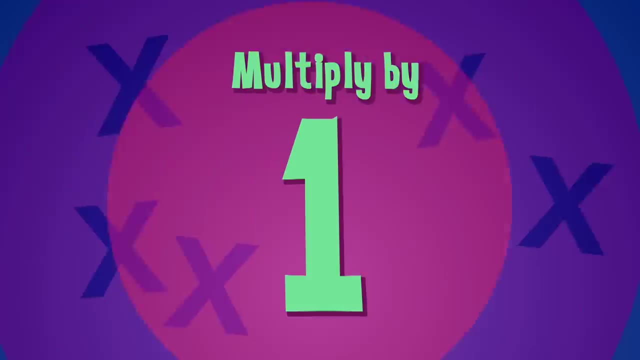 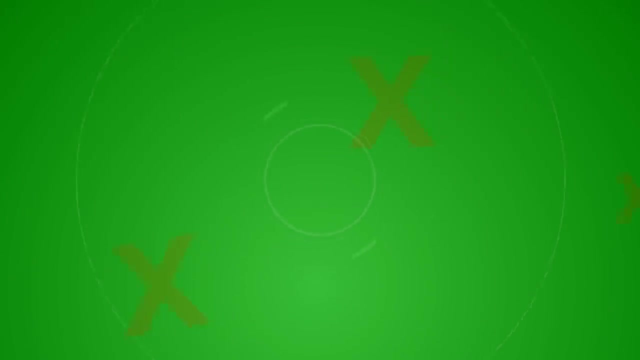 1,, 2,, 3,, 4,, 5,, 6,, 7,, 8,, 9,, 10,, 11,, 12.. Multiply by one Two times one is two. Two times two is four. Two times three is six. 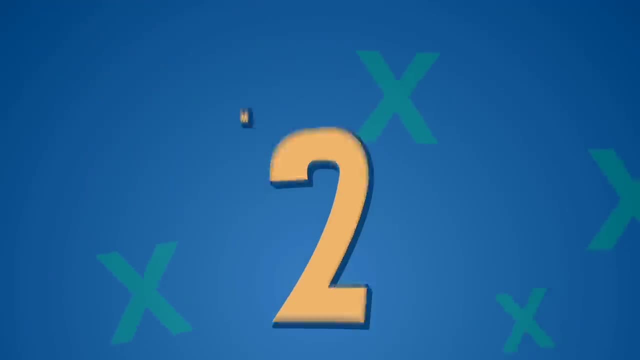 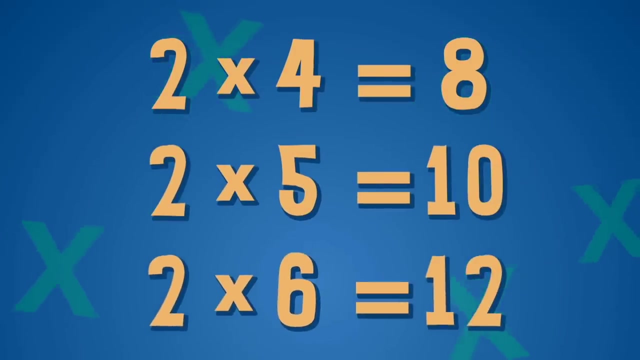 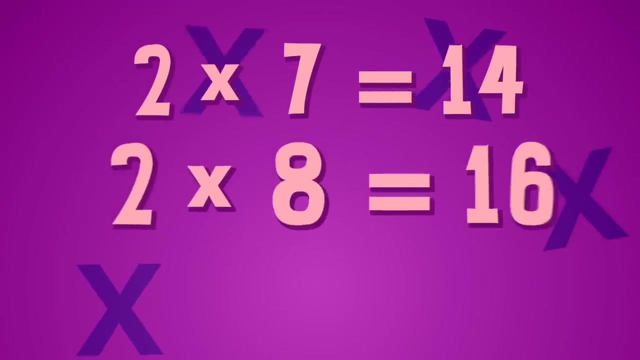 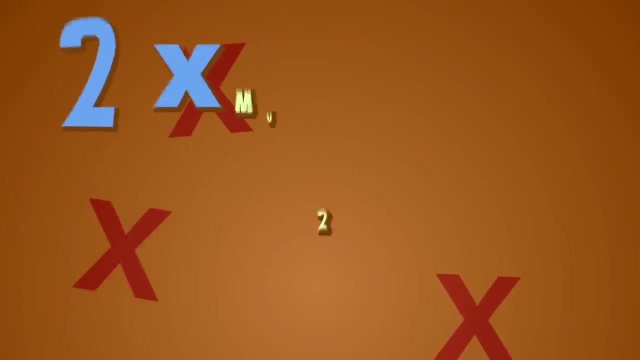 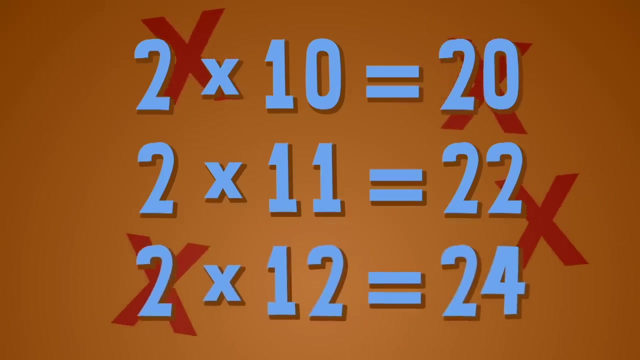 Multiply by two Two times four is eight. Two times five is ten. Two times six is twelve. Multiply by two Two times seven is fourteen. Two times eight is sixteen. Two times nine is eighteen. Multiply by two Two times ten is twenty. Two times eleven is twenty-two. Two times twelve is twenty-four. 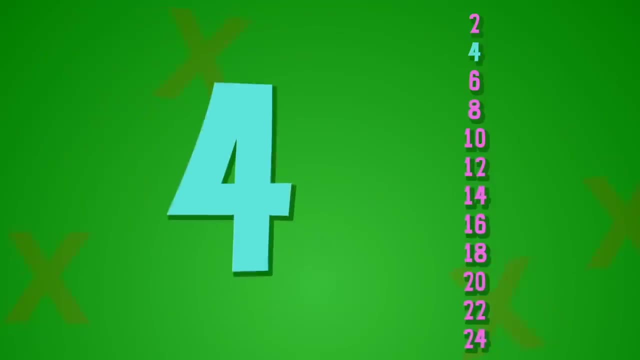 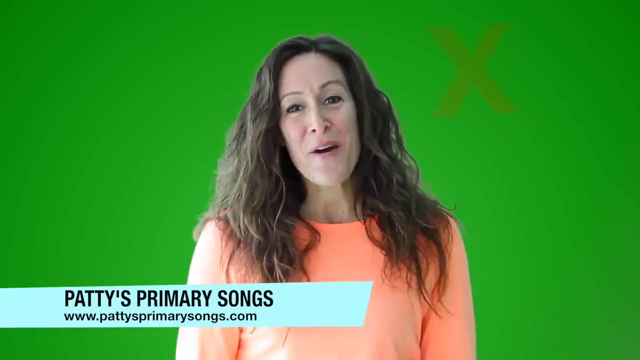 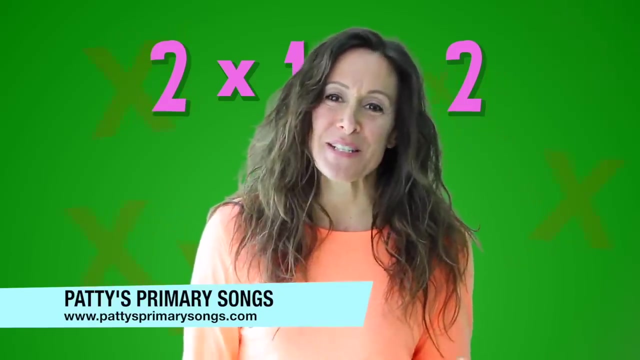 Multiply by two, Two, four, six, eight, ten, twelve, fourteen, sixteen, eighteen, twenty, twenty-two, twenty-four Multiply by two. Hi, If you liked that video, you can find the complete series and many more educational music videos at pattiesprimariesongscom. 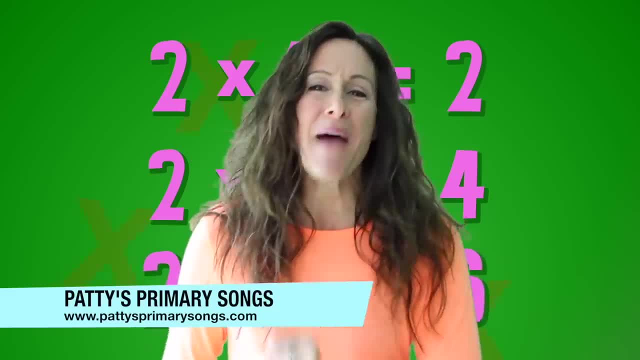 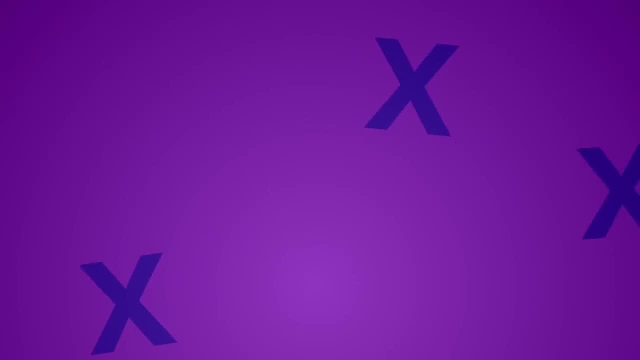 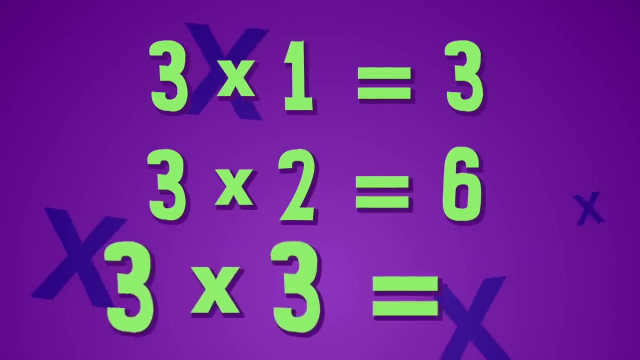 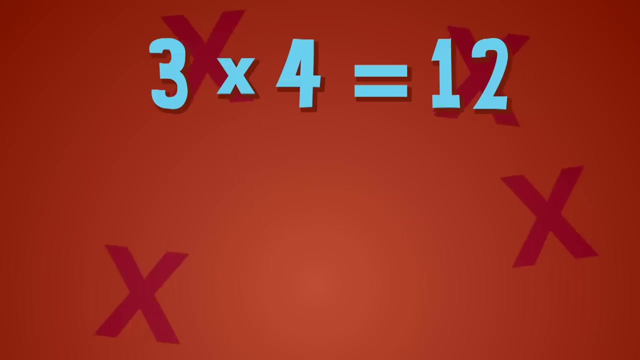 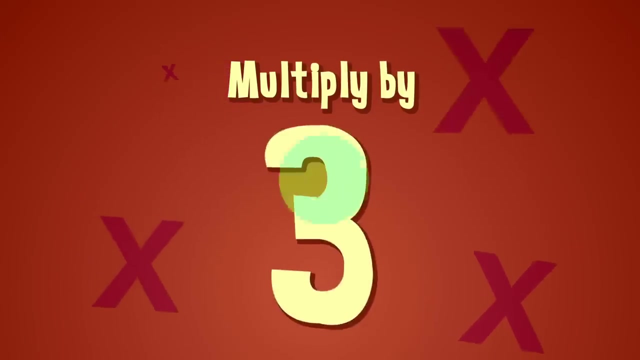 Just go to wwwpattiesprimariesongscom. Three times one is three. Three times two is six. Three times three is nine. Multiply by three, Three times four is twelve. Three times five is fifteen. Three times six is eighteen. Multiply by three, Three times seven is twenty-one. 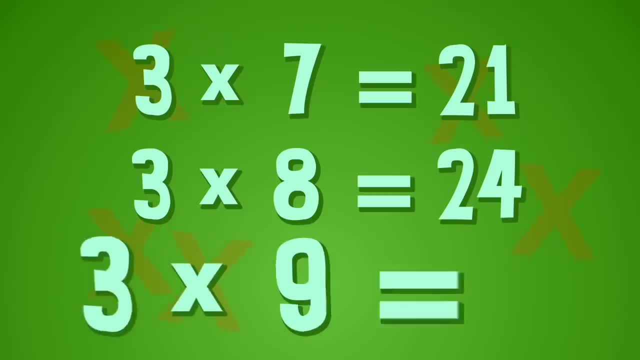 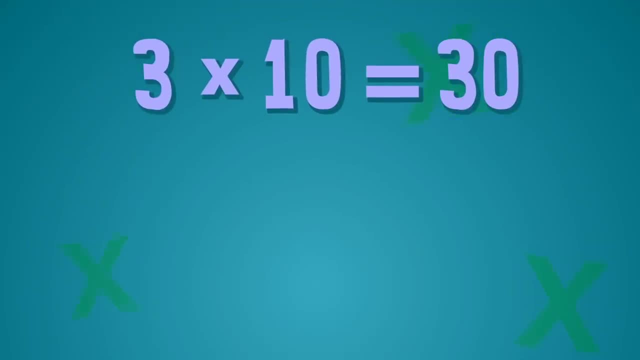 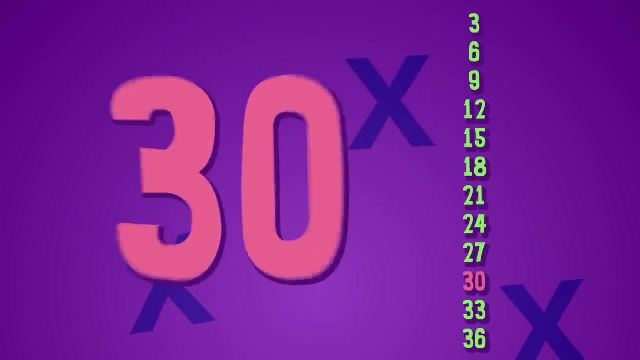 Three times eight is twenty-four. Three times nine is twenty-seven. Multiply by three, Three times ten is thirty. Three times eleven is thirty-three. Three times twelve is thirty-six. Multiply by three, Three, six, nine, twelve, fifteen, eighteen, twenty-one, twenty-four, twenty-seven, thirty, thirty-three, thirty-six. 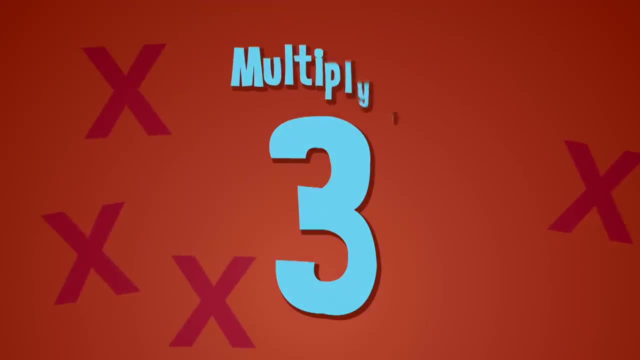 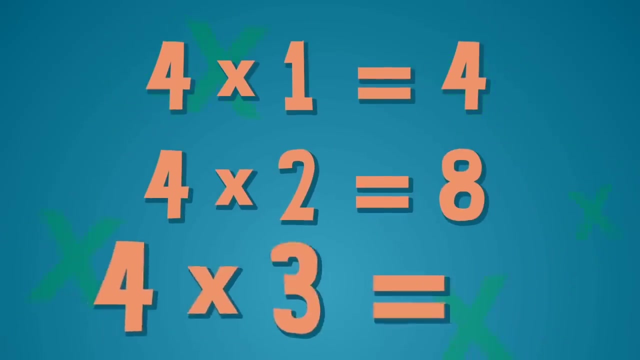 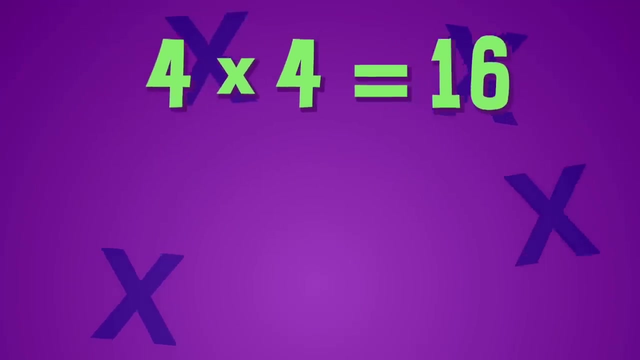 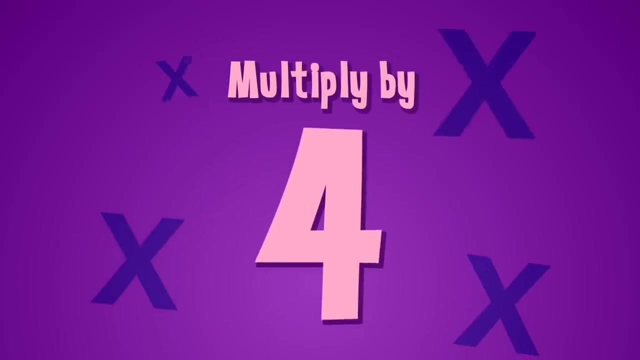 Multiply by three Four times one is four. Four times two is eight. Four times three is twelve. Multiply by four Four times four is sixteen. Four times five is twenty. Four times six is twenty-four. Multiply by four Four times seven is twenty-eight. Four times eight is thirty-two. 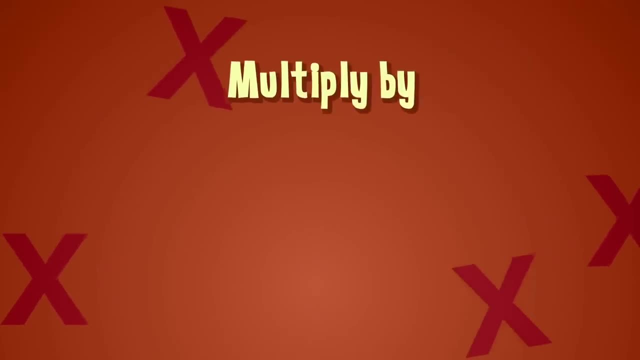 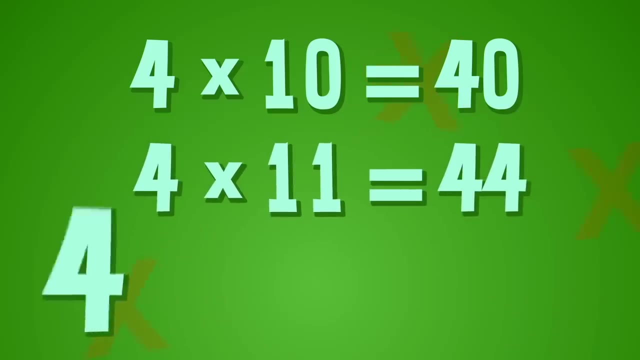 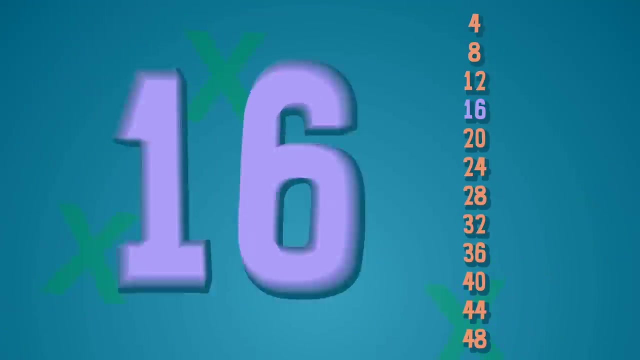 Four times nine is thirty-six Multiply by four. Four times ten is forty. Four times eleven is forty-four. Four times twelve is forty-eight Multiply by four, Four, eight, twelve, sixteen, twenty, Twenty-four, twenty-eight, thirty-two, thirty-six, Forty, forty-four, forty-eight. 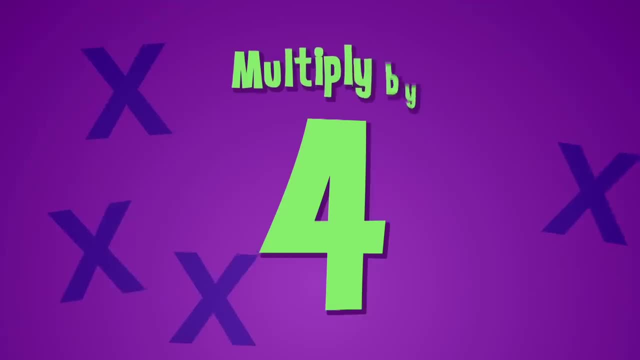 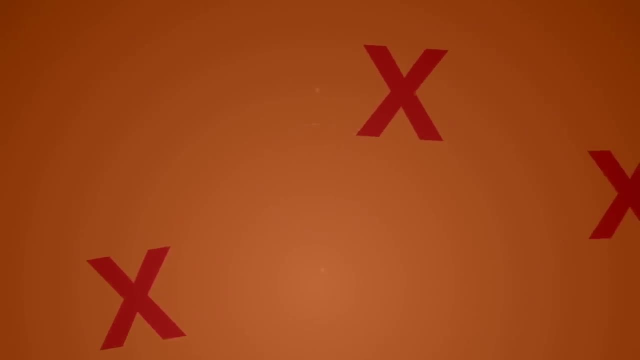 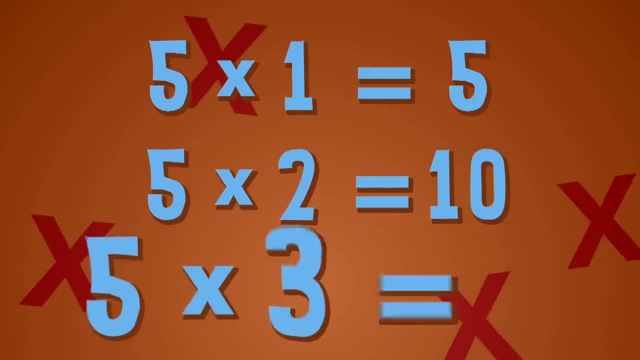 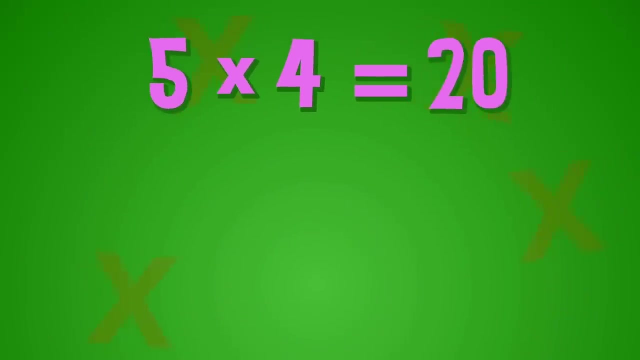 Multiply by four, Five times one is five. Five times two is ten. Five times three is fifteen. Multiply by five, Five times four is twenty. Five times five is twenty-five. Five times six is thirty. Multiply by five, Five times seven is thirty-five. Five times eight is forty. 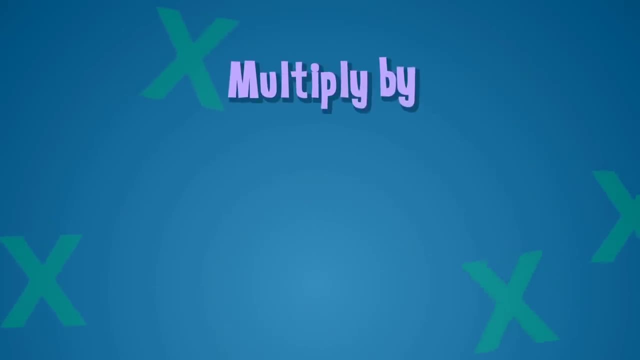 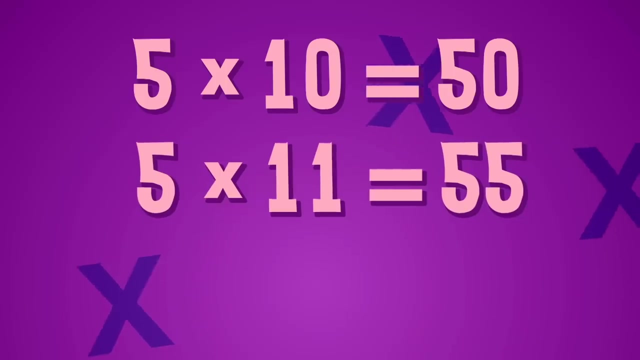 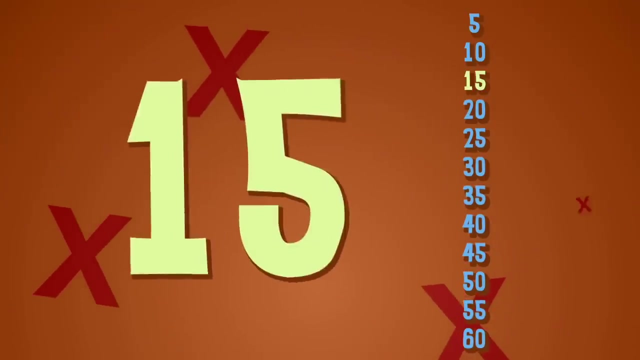 Five times nine is forty-five. Multiply by five. Five times ten is fifty. Five times eleven is fifty-five. Five times twelve is sixty, Multiply by five, Five, ten, fifteen, twenty, Twenty-five, thirty, thirty-five, forty, Forty-five, fifty, fifty-five, sixty. 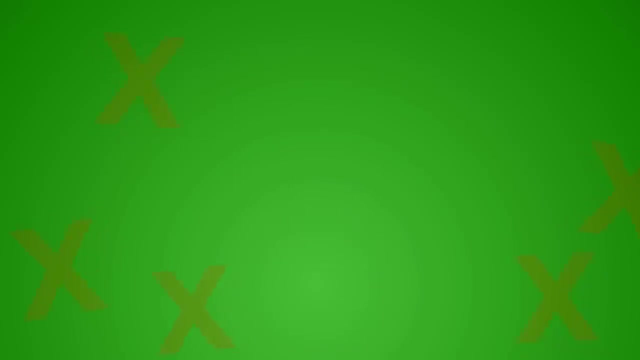 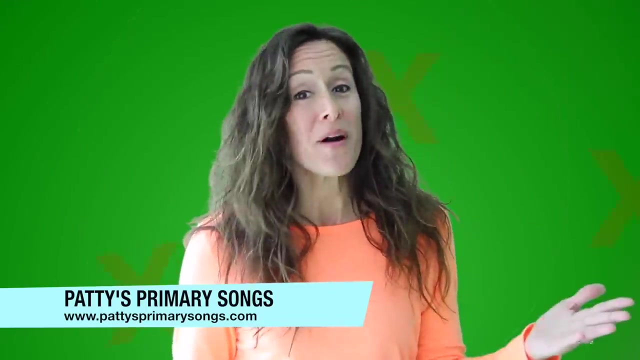 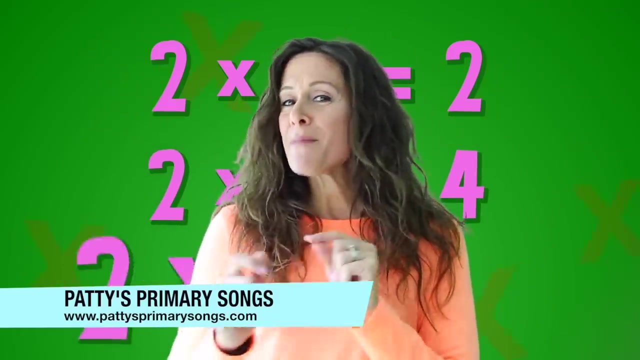 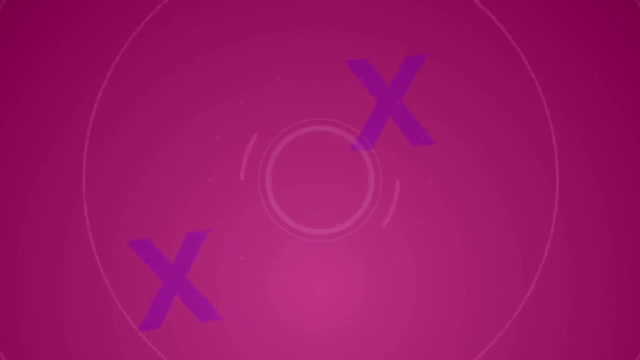 Multiply by five. If you liked that video, you can find the complete series and many more educational music videos at Paddy'sPrimarySongscom. Just go to wwwPaddy'sPrimarySongscom. Six times one is six. Six times two is twelve. Six times three is eighteen. 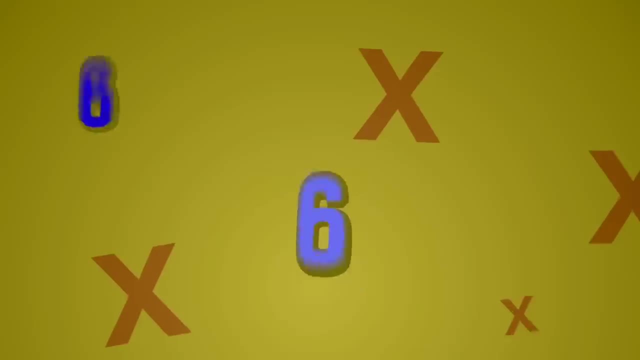 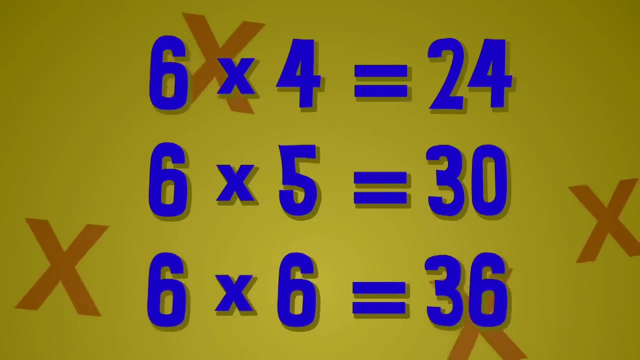 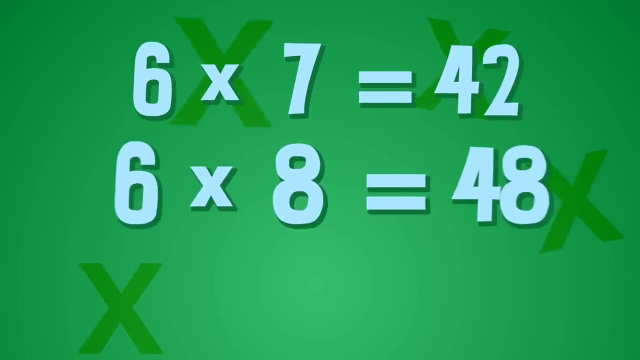 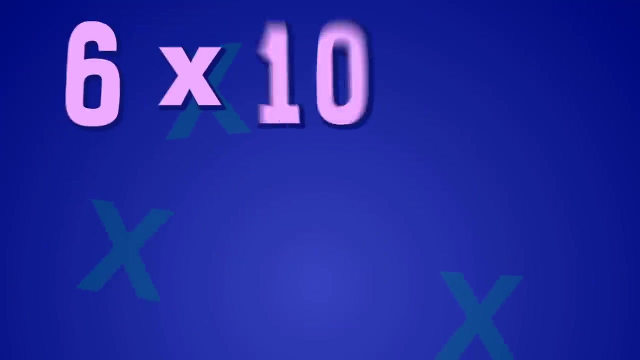 Multiply by six, 6 times 4 is 24,. 6 times 5 is 30,. 6 times 6 is 36,. multiply by 6, 6 times 7 is 42,. 6 times 8 is 48,. 6 times 9 is 54,. multiply by 6, 6 times 10 is 60,. 6 times 11 is 66,. 6 times 12 is 72,. 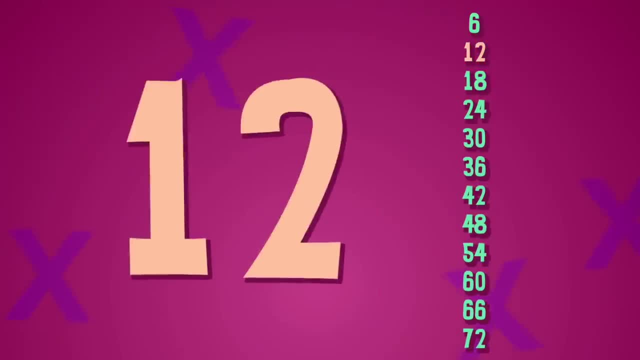 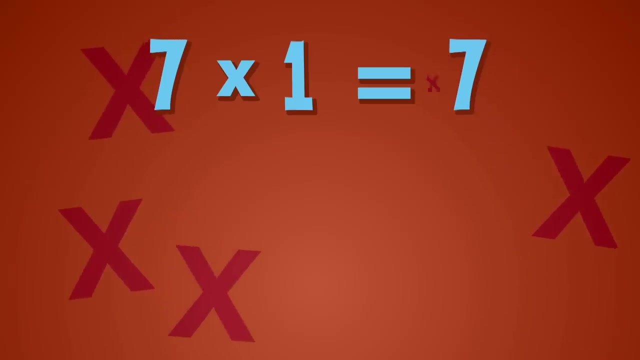 multiply by 6,, 6,, 12,, 18,, 24,, 30,, 36,, 42,, 48,, 54,, 60,, 66,, 72,. multiply by 6.. 7 times 1 is 7,, 7 times 2 is 14,. 7 times 3 is 21,. 7 times 3 is 21,. 7 times 2 is 14,. 7 times 3 is 21,. 7 times 1 is 7,. 7 times 2 is 14,. 7 times 3 is 21,. 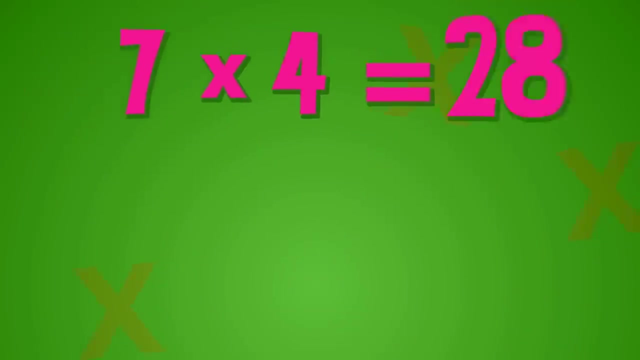 multiplied by 7, 7 times 4 is 28, 7 times 5 is 35, 7 times 6 is 42. multiplied by 7, 7 times 7 is 49, 7 times 8 is 56, 7 times 9 is 63. 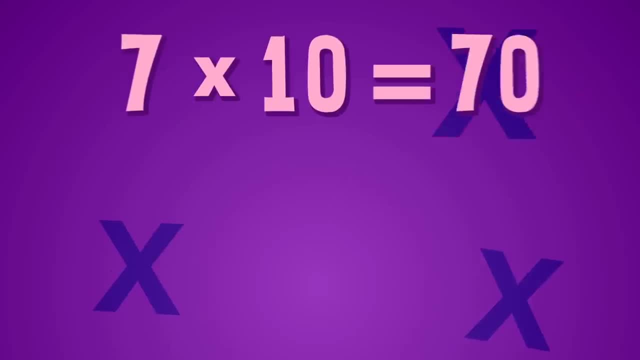 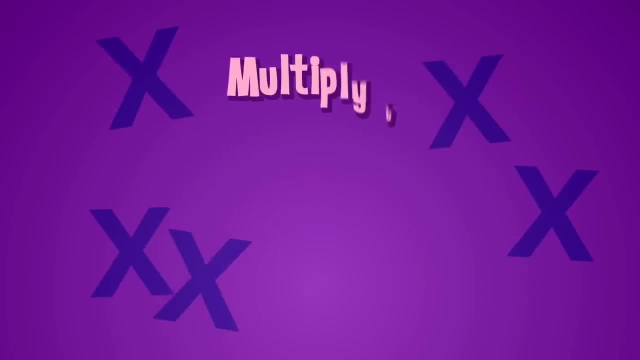 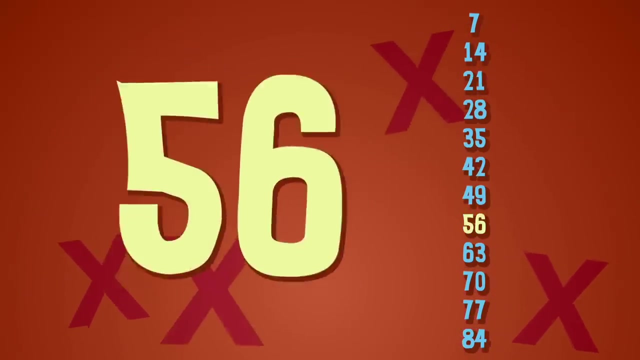 multiplied by 7, 7 times 10 is 70, 7 times 11 is 77. 7 times 12 is 84. multiplied by 7, 7,, 14,, 21,, 28,, 35,, 42,, 49,, 56,, 63,, 70,, 77,, 84. 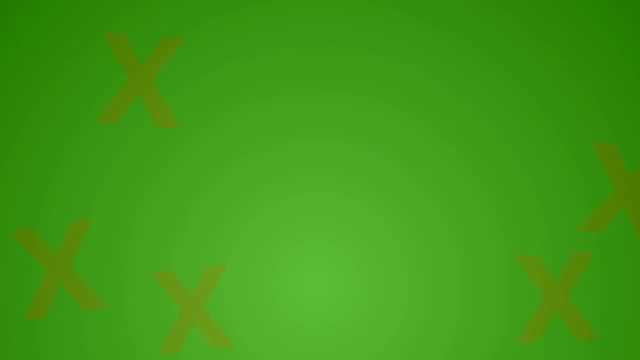 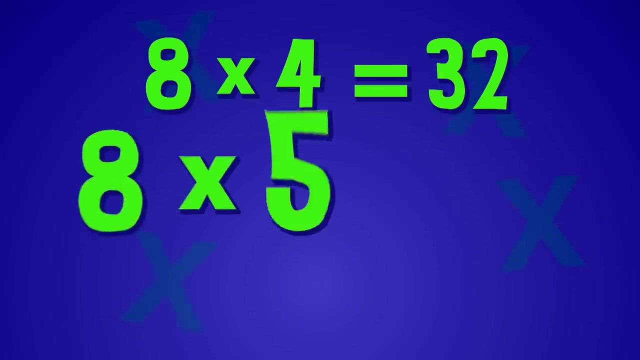 multiplied by 7, 8 times 1 is 8, 8 times 2 is 16. 8 times 3 is 24. multiplied by 8, 8 times 4 is 32. 8 times 5 is 40. 8 times 6 is 48. 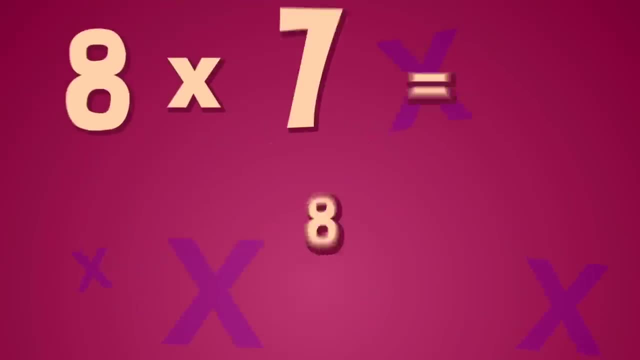 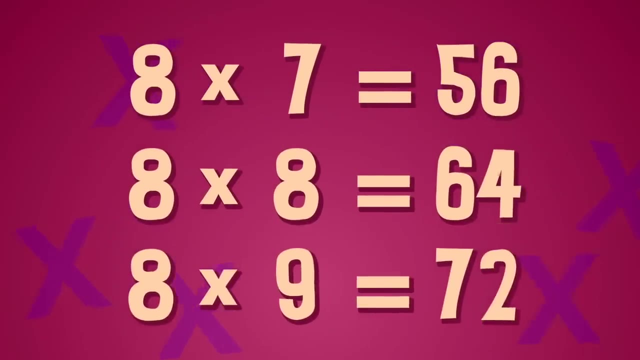 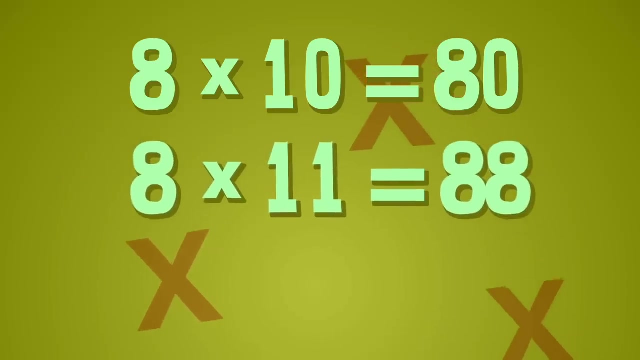 multiplied by 8, 8 times 7 is 56. 8 times 8 is 64. 8 times 9 is 72. multiplied by 8, 8 times 10 is 80, 8 times 11 is 88. 8 times 12 is 96. 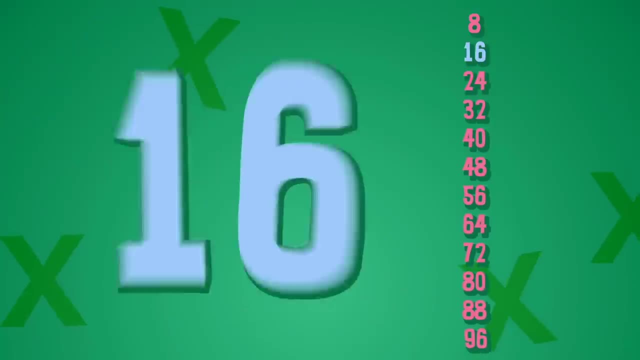 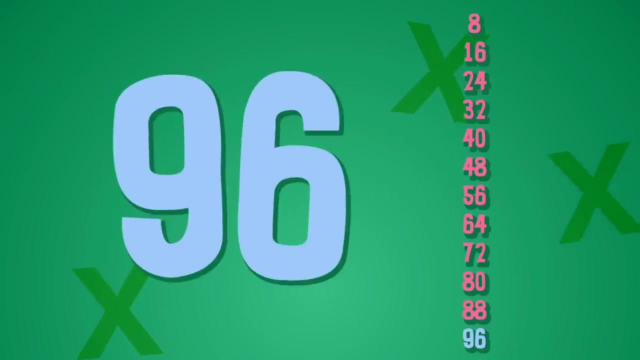 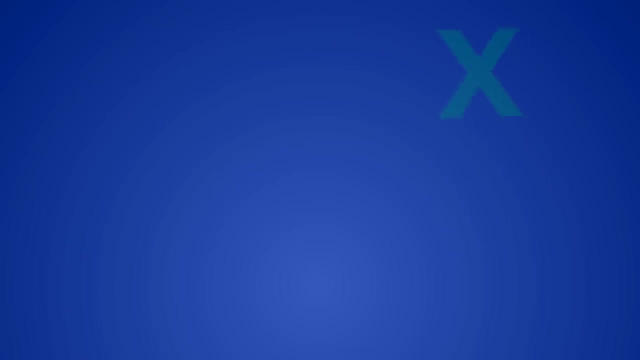 multiplied by 8, 8,, 16,, 24,, 32,, 40,, 48,, 56,, 64,, 72,, 80,, 88,, 96, multiplied by 8, 9 times 1, is 9. 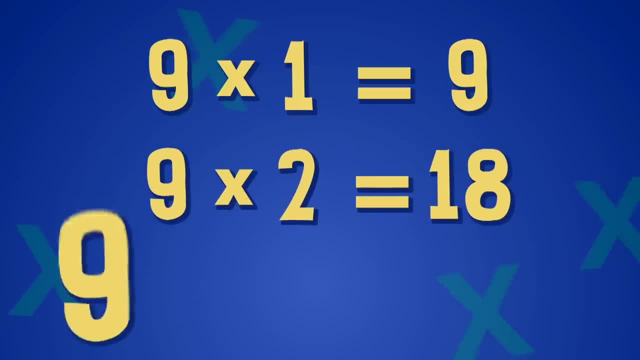 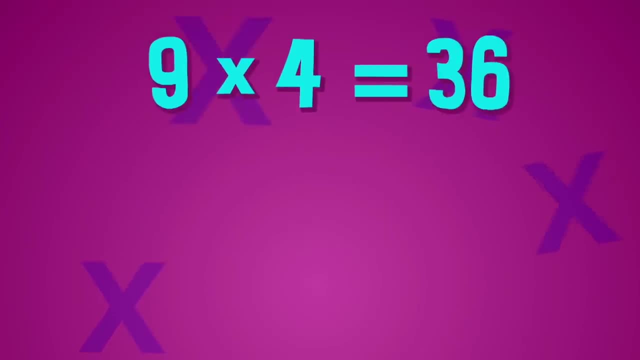 9 times 2 is 18. 9 times 3 is 27. multiplied by 9. 9 times 4 is 36. 9 times 5 is 45. 9 times 6 is 54. multiplied by 9. 9 times 7 is 63. 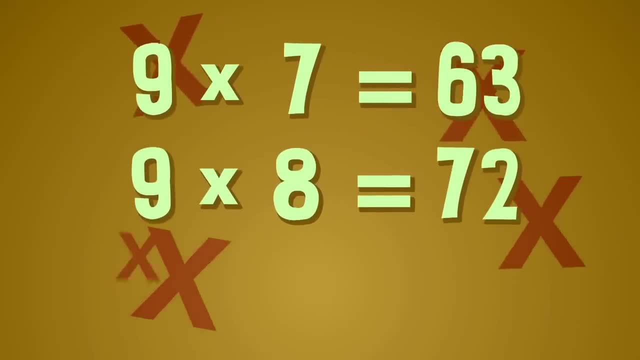 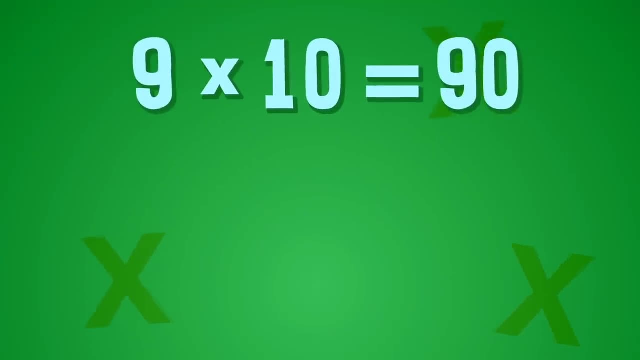 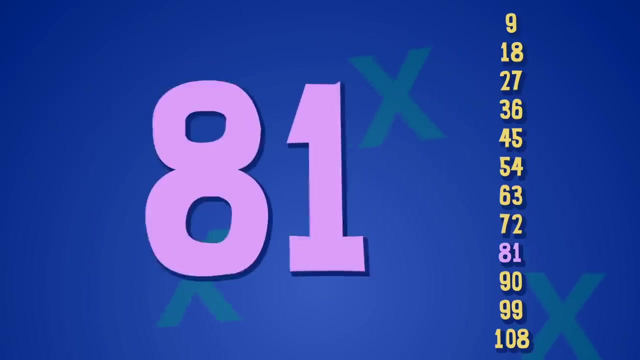 9 times 8 is 72. 9 times 9 is 81, multiplied by 9. 9 times 10 is 90. 9 times 11 is 99. 9 times 12 is 108 multiplied by 9, 9,, 18,, 27,, 36,, 45,, 54,, 63,, 72,, 81,, 90,, 99,, 108. 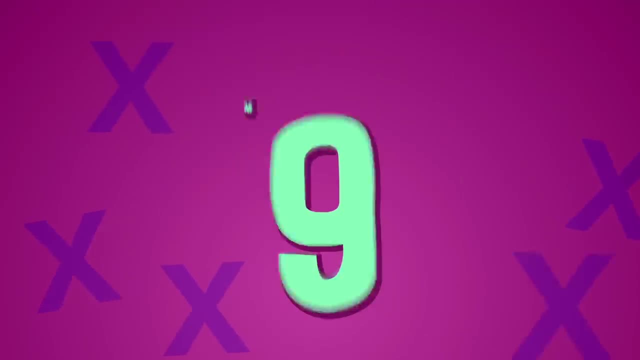 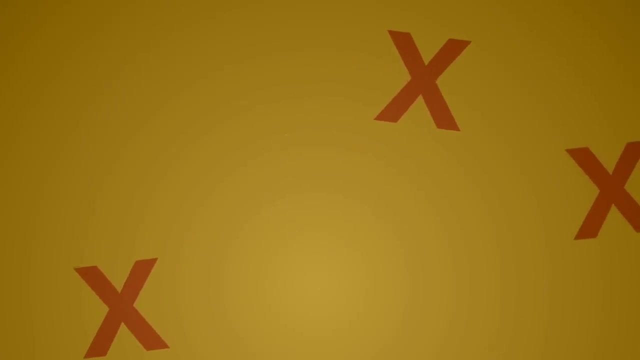 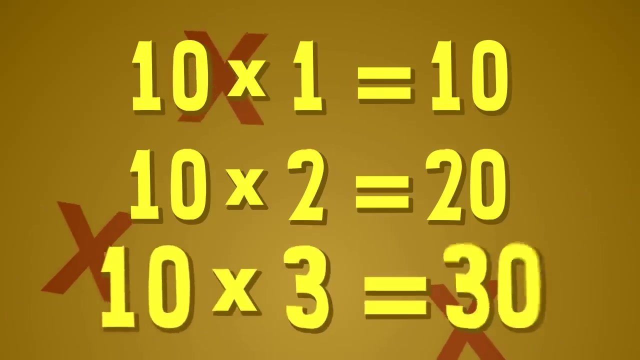 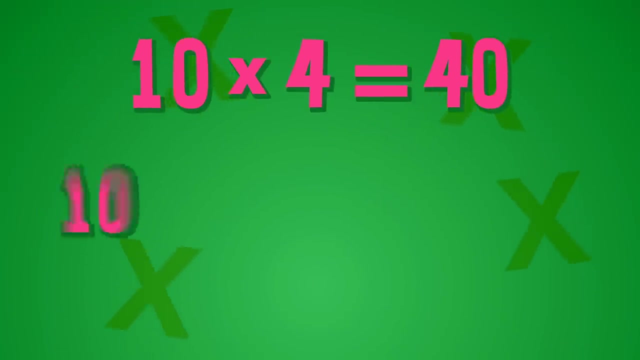 multiplied by 9: 10 times 1 is 10, 10 times 2 is 20. 10 times 3 is 30. multiplied by 10, 10 times 4, is 40. 10 times 5 is 50. 10 times 6 is 60. 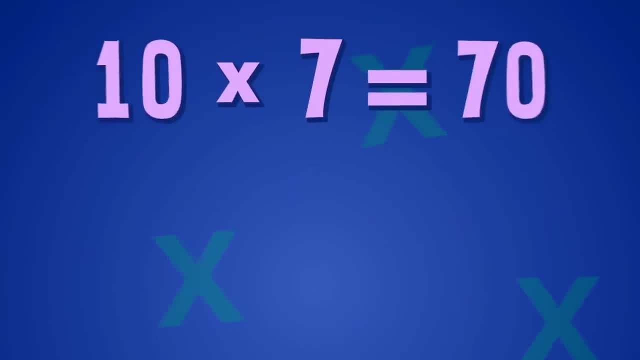 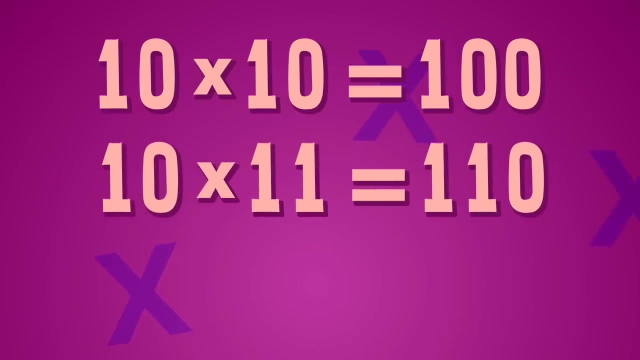 multiplied by 10: 10 times 7 is 70. 10 times 8 is 80. 10 times 9 is 90. multiply by 10: 10 times 10, is 100. 10 times 11 is 110. 10 times 12 is 120. 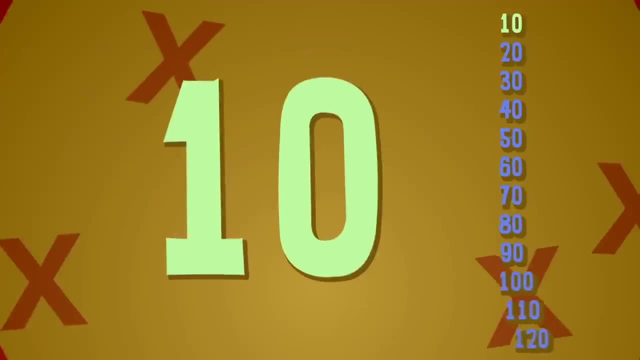 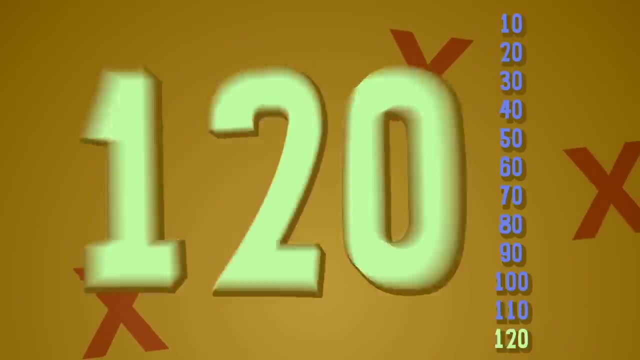 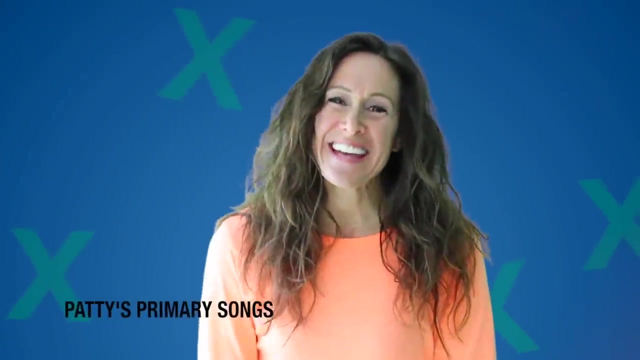 multiply by 10. 10,, 20,, 30,, 40,, 50,, 60,, 70,, 80,, 90,, 100,, 110,, 120. multiply by 10. Hi, If you liked that video, you can find the complete series. 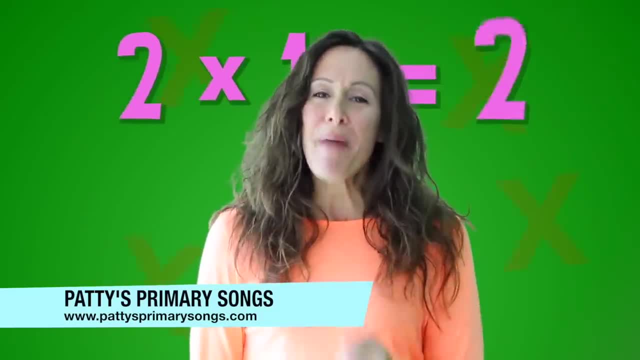 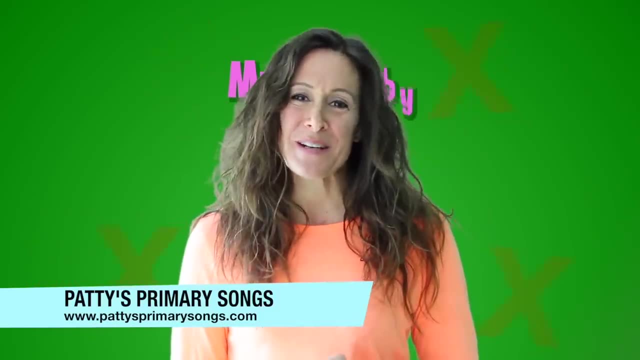 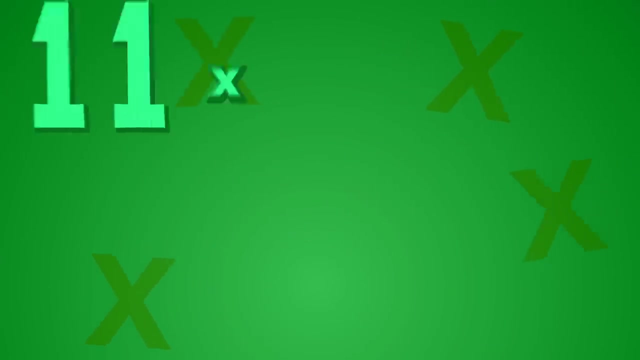 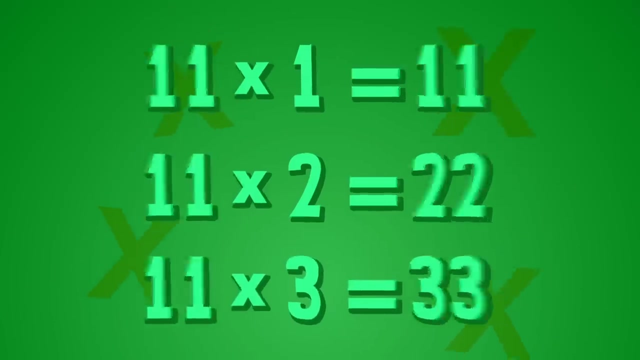 and many more educational music videos at pattiesprimariesongscom. Just go to wwwpattiesprimariesongscom. 11 times 1 is 11. 11 times 2 is 22. 11 times 3 is 33 multiplied by 11. 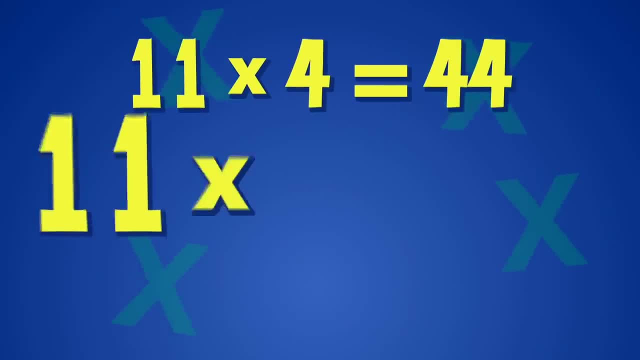 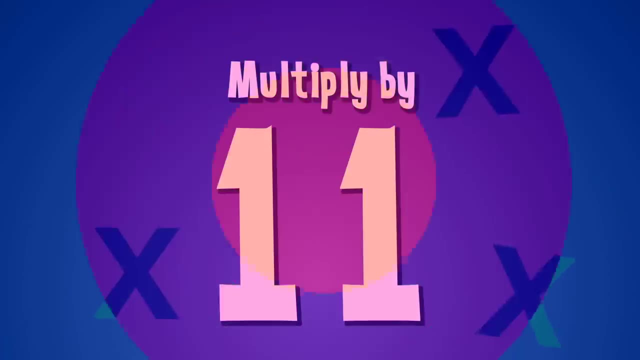 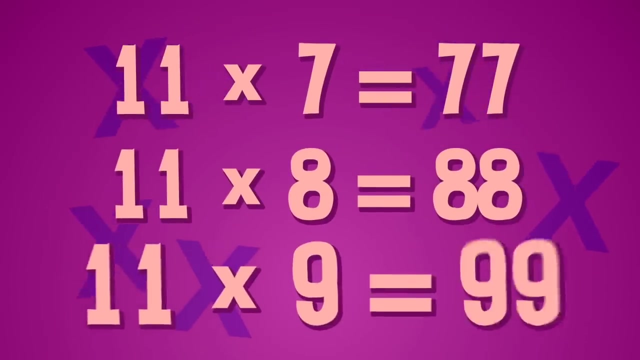 11 times 4 is 44. 11 times 5 is 55. 11 times 6 is 66. multiplied by 11, 11 times 7 is 77. 11 times 8 is 88. 11 times 9 is 99. 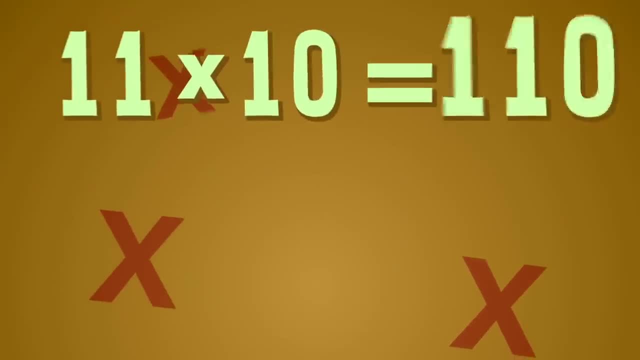 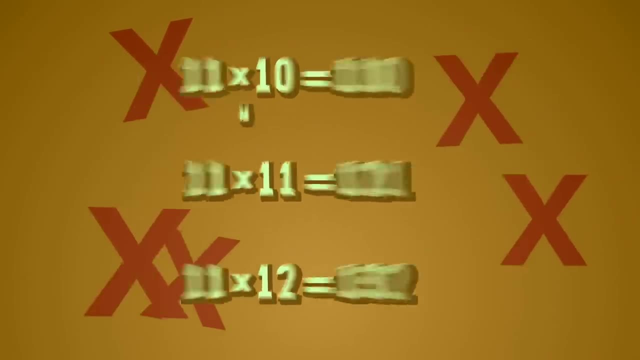 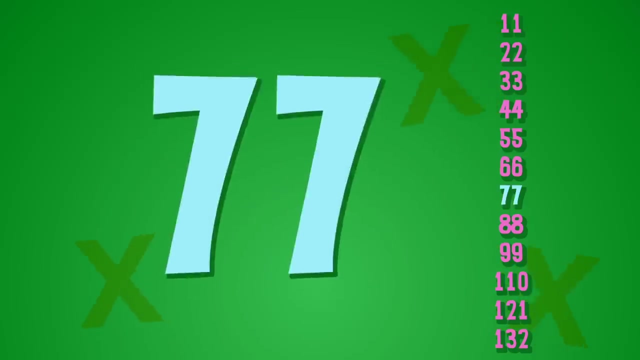 multiplied by 11. 11 times 10 is 110. 11 times 11 is 121. 11 times 12 is 132. multiplied by 11, 11,, 22,, 33,, 44,, 55,, 66,, 77,, 88,, 99,, 110,, 121,, 132.